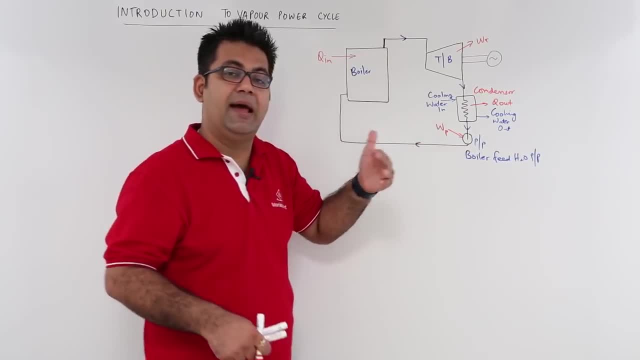 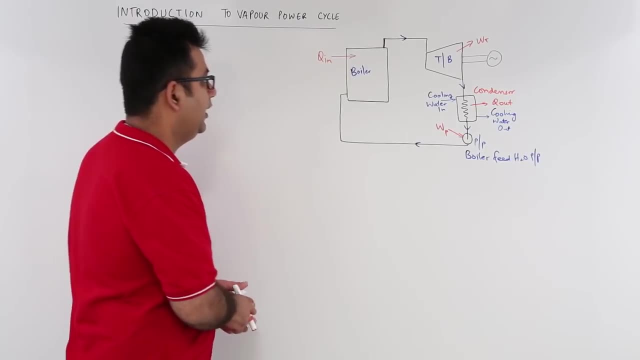 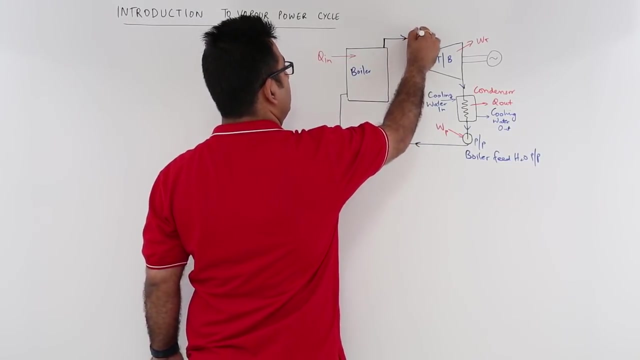 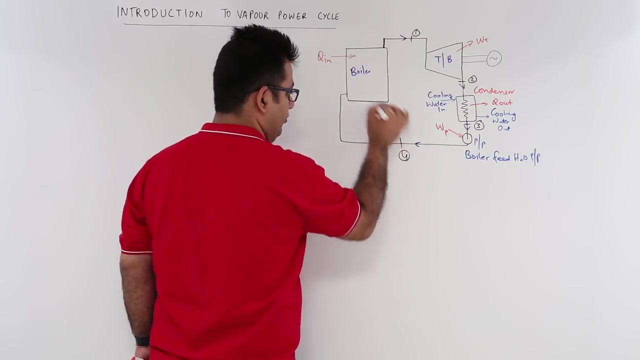 output minus input. ok, your input work has to be less as compared to the output work, otherwise the you know cycle would be impractical to run, right? so if you look at this, let us say this is state 1, this is state 2, this is state 3 and this is state 4. ok, so from 1 to 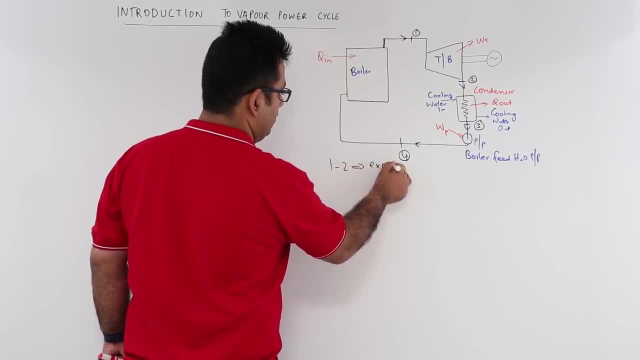 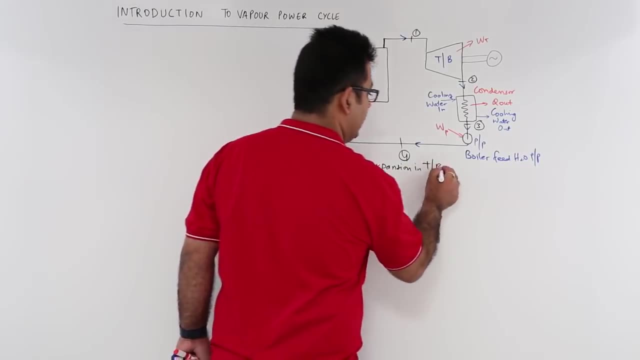 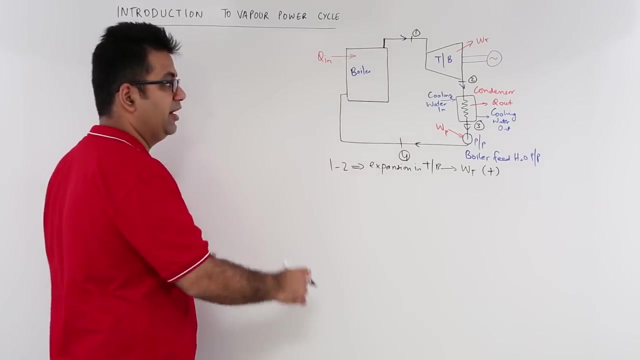 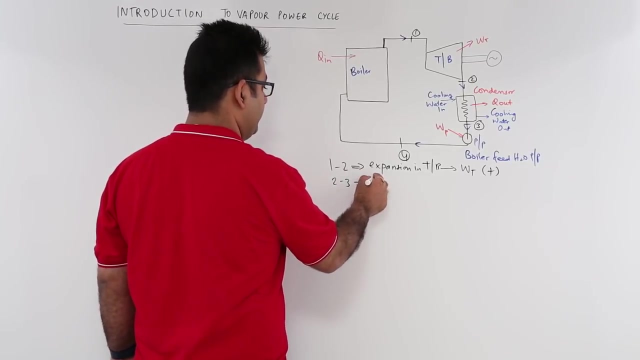 2. you have expansion and turbine. ok ok, ok, ok, ok. this expansion in turbine gives us turbine work. this turbine work is a positive value because we are getting work out of the system. then, 2 to 3, 2 to 3: this would be heat rejection. 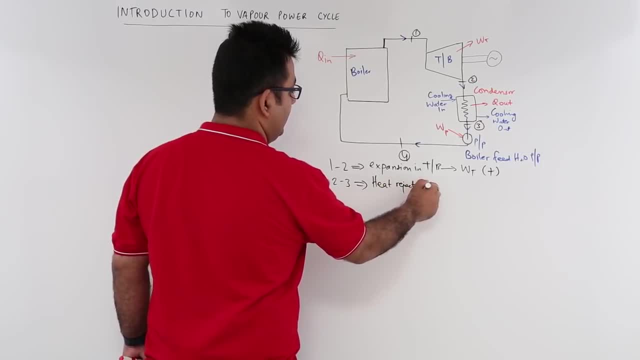 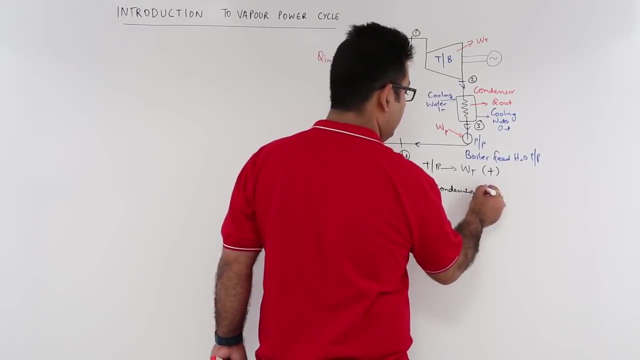 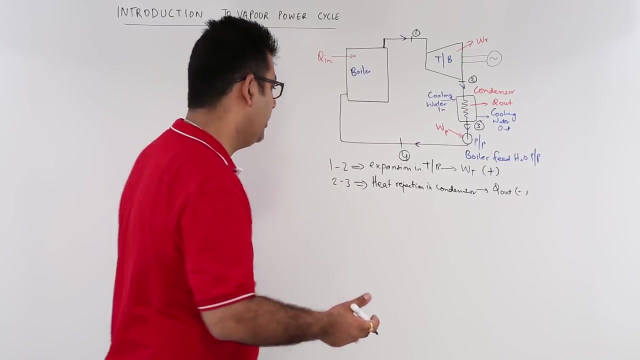 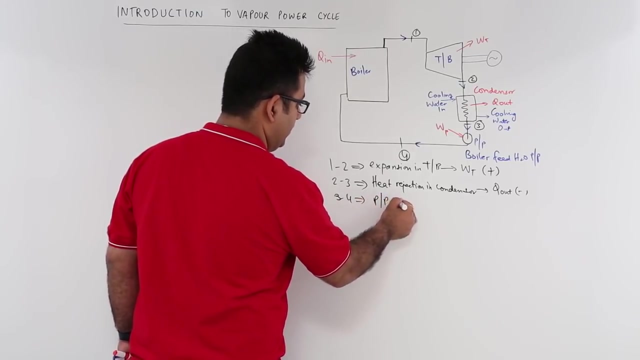 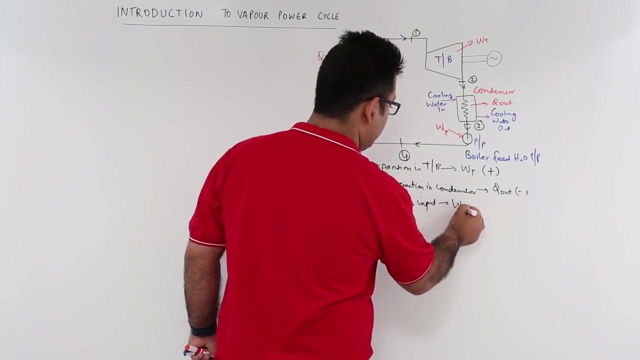 ok, this would be heat rejection in condenser. ok, and this would be q out and because it is going out of the system, this would be negative. ok, 3 to 4. 3 to 4 would be pump work input. ok, and this is work input. we are providing work to the system, so this becomes a negative quantity. 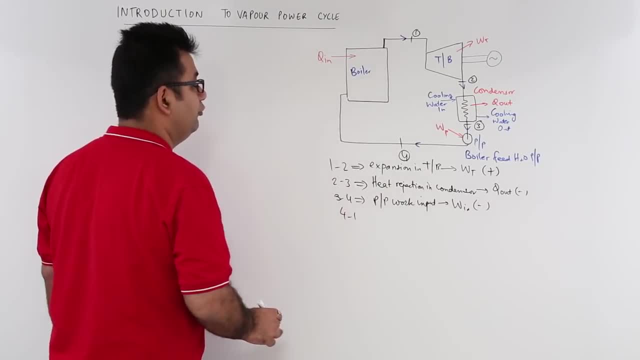 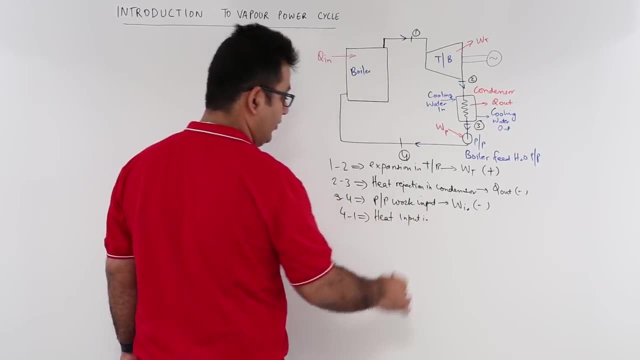 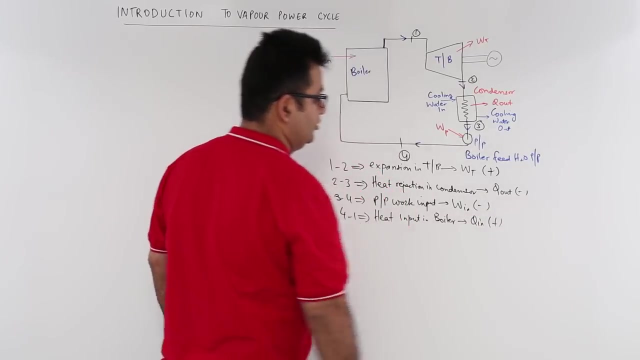 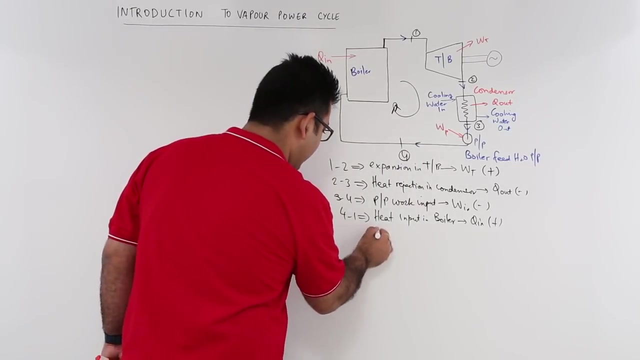 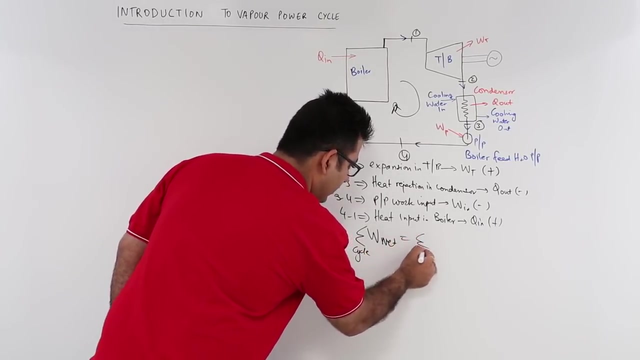 and then, from 4 to 1, we have heat input in boiler, so this becomes q in and this is positive. ok now, because it is a cycle. it is a cycle, ok, so net work done. net work done for a cycle is equal to the net heat interaction for the. 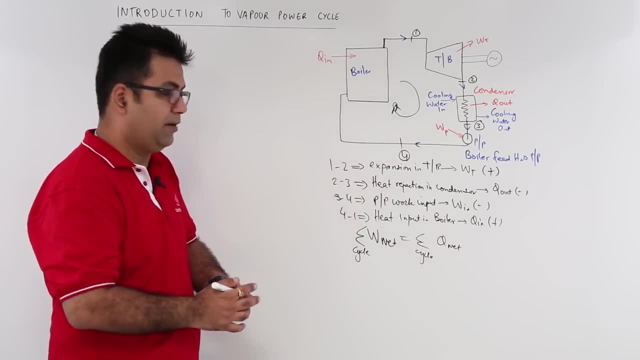 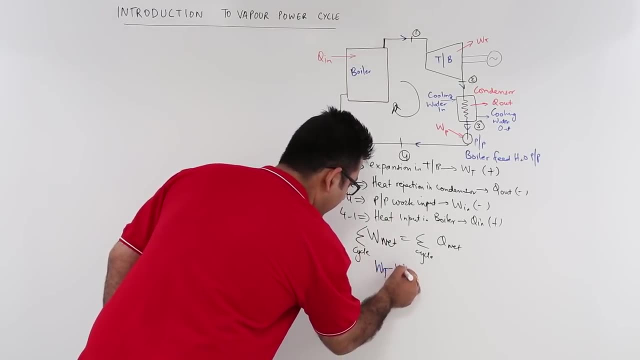 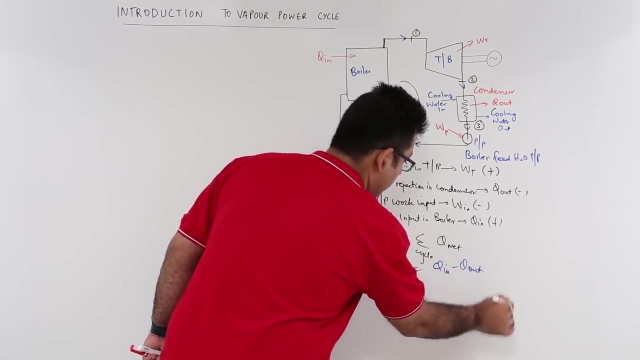 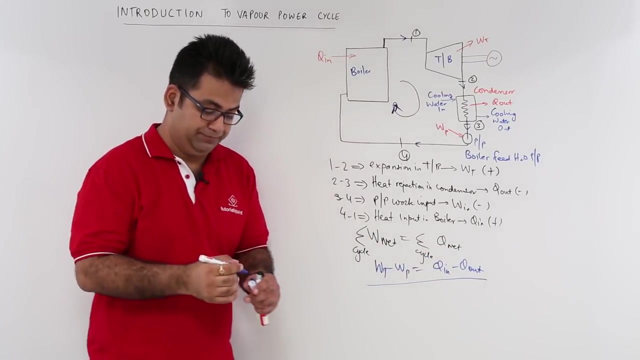 cycle. so this is as per the first law of thermodynamics for a cycle. so the net work for this would be wt minus wp, and this is equal to q in, equal to Q in minus Q out. so this equation is true for any cycle. alright, now this is: 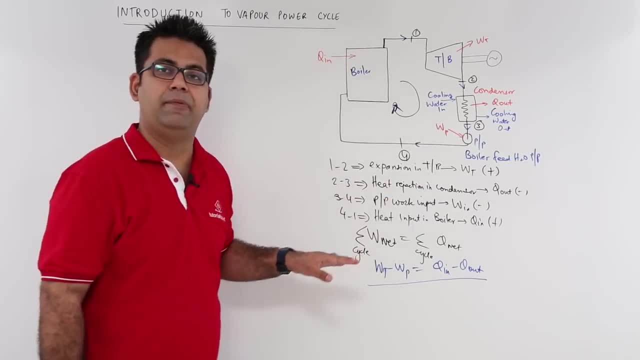 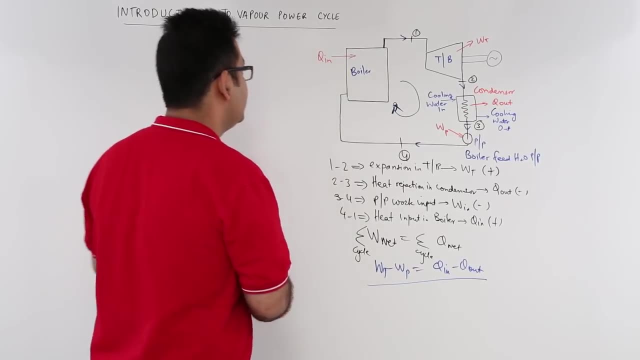 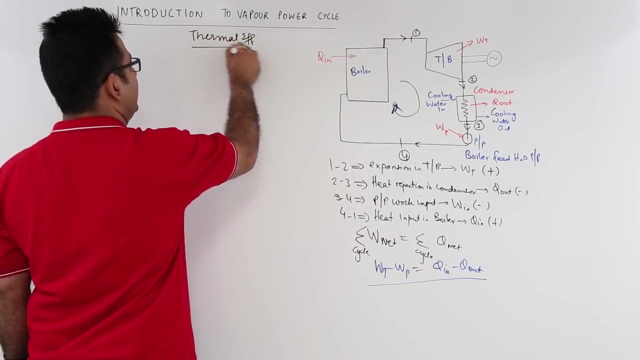 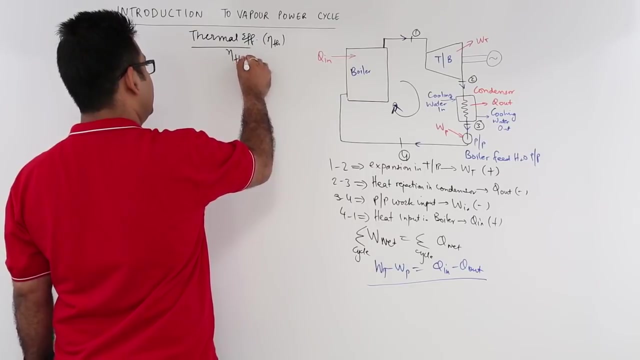 very brief introduction on how a steam vapor power plant looks. now let's talk about some important term for this. the very first term is the thermal efficiency. thermal efficiency- and we all know what it is- It is the net work output upon heat input. so that is eta. Th is equal to net work output. 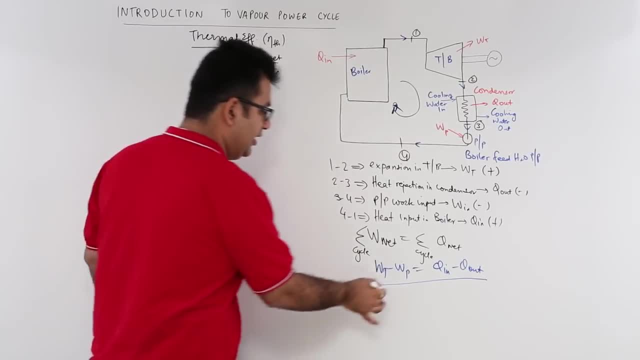 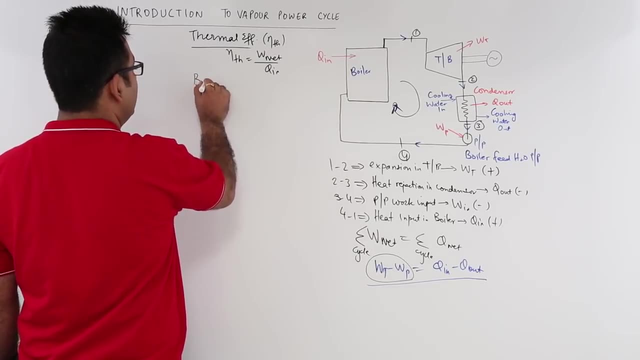 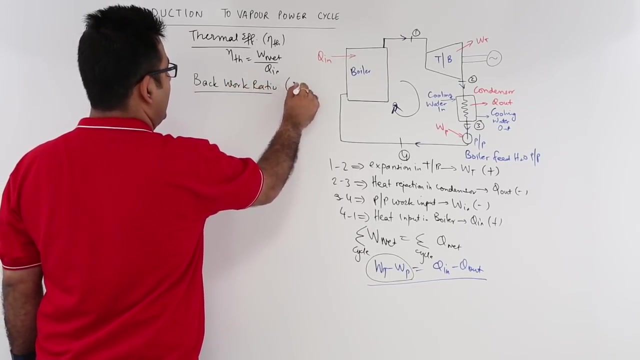 upon heat input, which is net work output as Wt minus Wp. the second one, the second term, is the back work ratio. this is R B W. So R Bw of p is the beforehand method, which is also known as thermal efficiency reactor strainer. 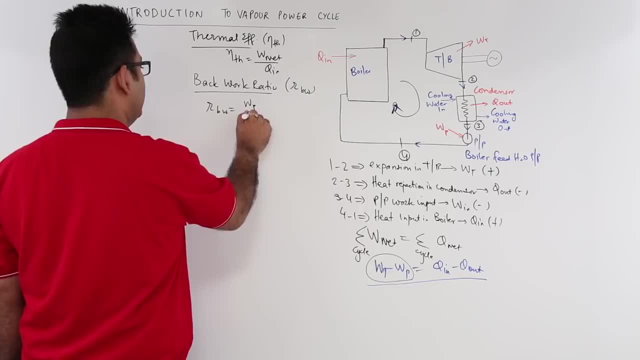 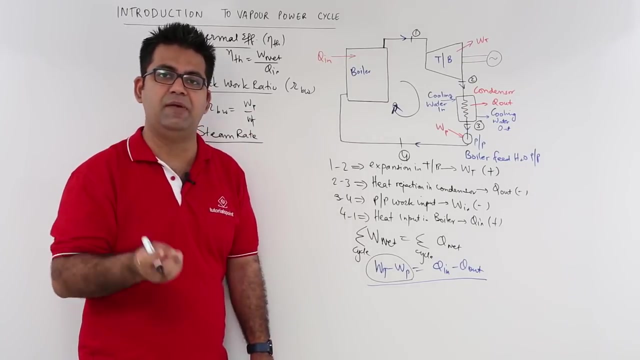 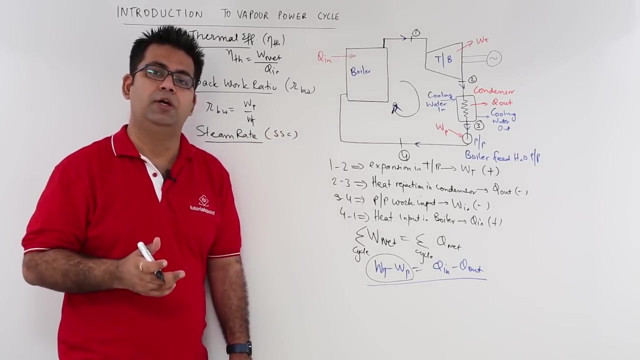 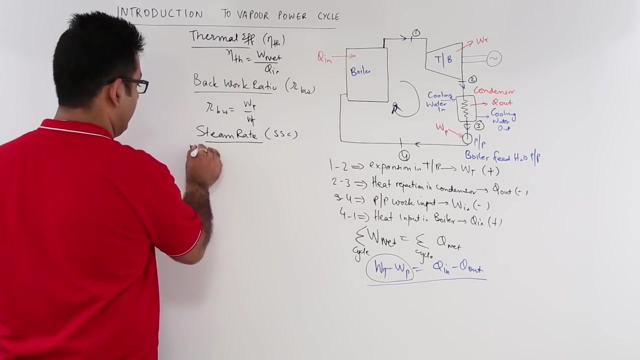 So the second one brings us the… pw. this is the ratio of pump work upon turbine work. the next ratio, or the next term, is steam rate. steam rate is also known as the specific steam consumption, ssc, and this is the amount of steam required to produce 1 kilowatt hour of power. so this is the mass of steam needed. 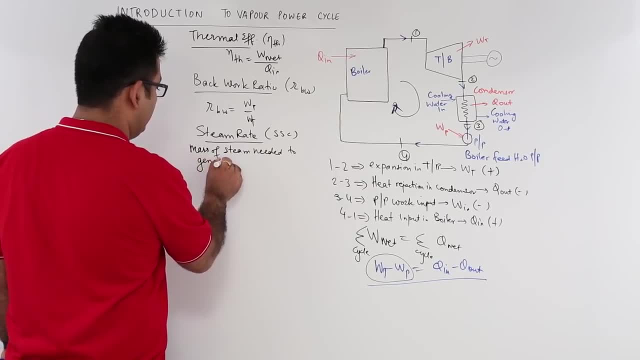 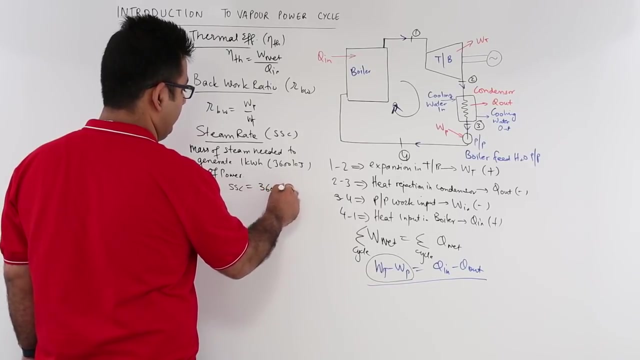 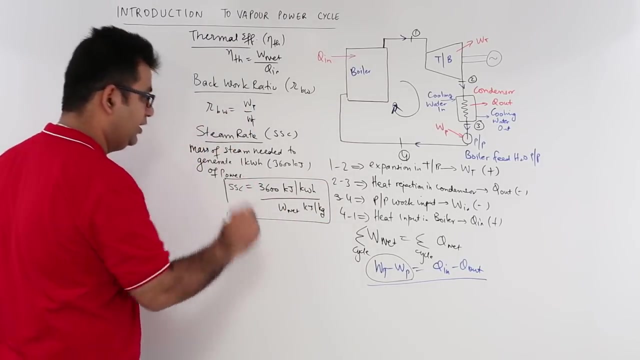 to generate, to generate 1 kilowatt hour. or it is also 3600 kilojoules of power. so this is the mass of power. ok, and the mathematical relation to find out: steam rate is 3600 kilojoules per kilowatt hour upon net work, which is in kilojoules per kg. so this is how we find out. 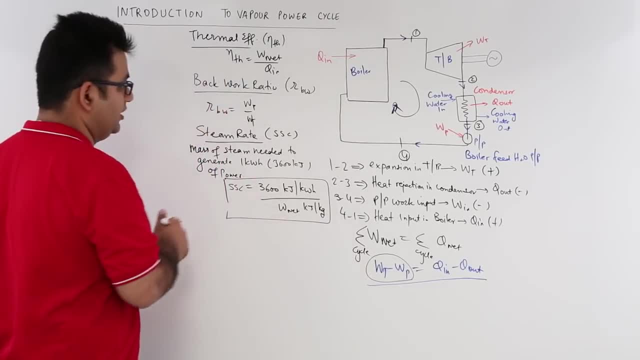 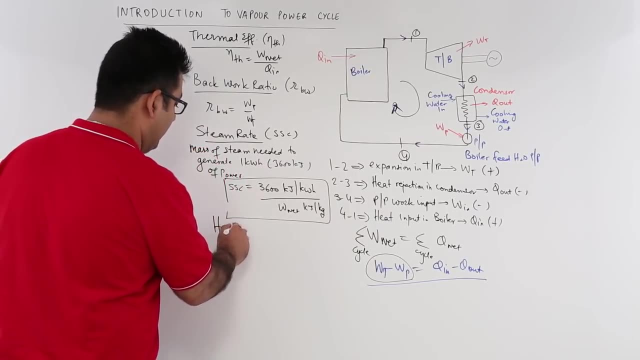 the specific steam consumption. the last term that we will be learning about is the mass of steam. the last term that we will be learning about the vapor power cycle is the heat rate, heat rate. and what is heat rate? heat rate is the amount of heat needed to produce 1 kilowatt.